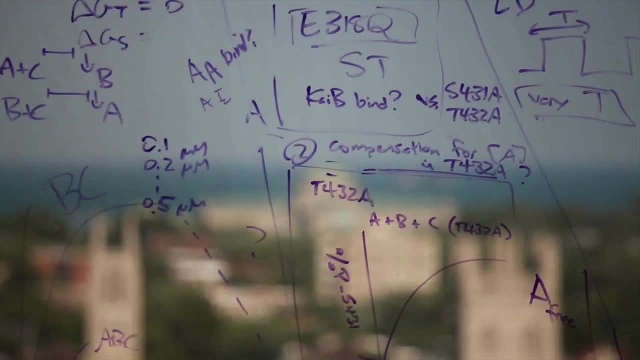 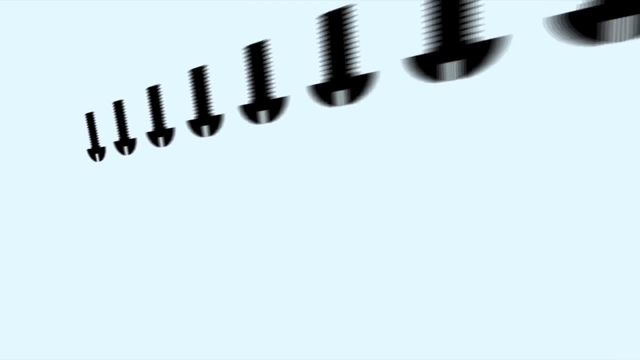 Systems biology involves theory, computation and experiment. One way you can think about systems biology is in the context of engineering. So if you want to understand what keeps a plane in the air, you can't just look at one bolt at a time. 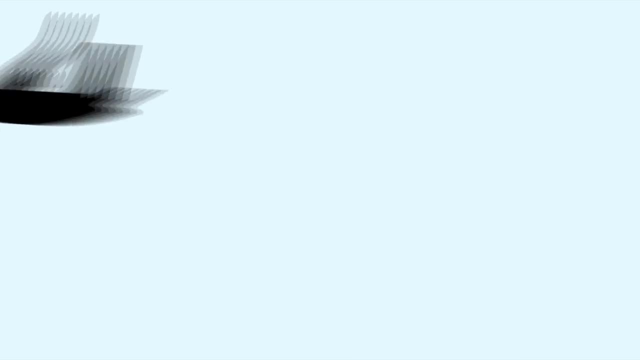 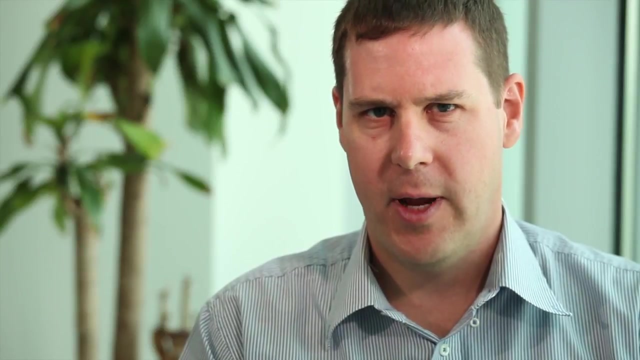 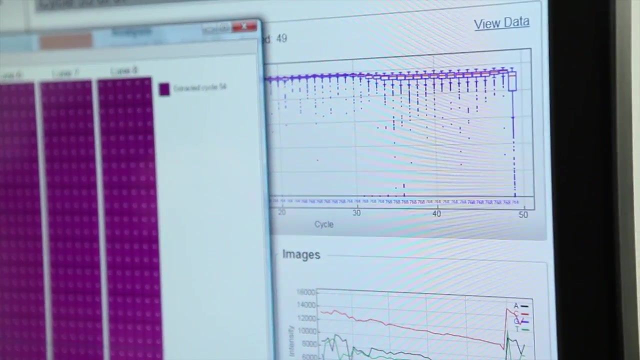 You have to look at the entire system together And you have to have a framework that allows you to make predictions about what is going to happen under different conditions. That's what biologists do. They make a model of a very complex system and they make predictions about what's going to happen to that system. 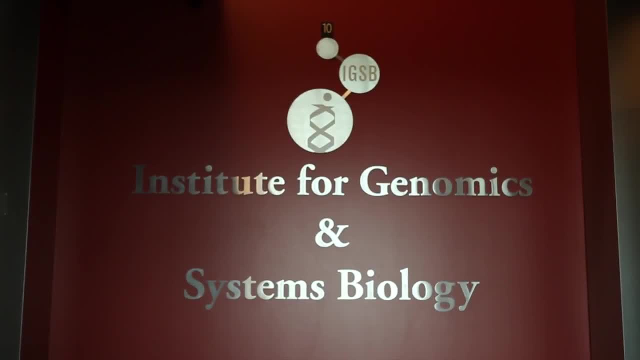 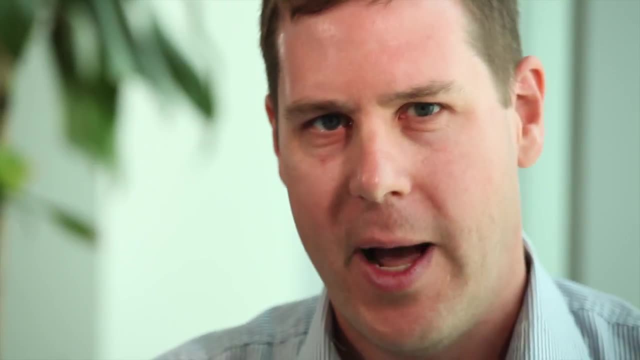 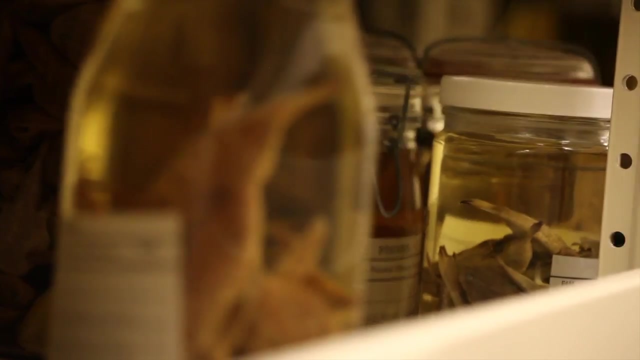 when you change a part of it. And the systems that biologists study are not bolts, they're not screws, but they're genes, they're proteins, they're RNAs, they're biomolecules that fit together into very complex, complex networks that create cells and organs and animals. 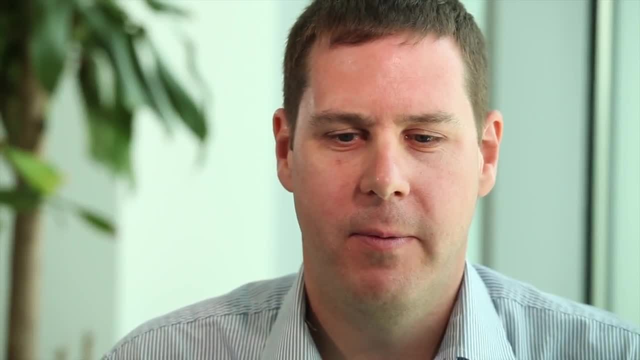 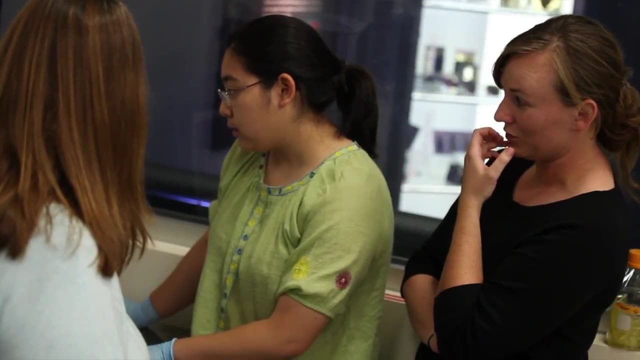 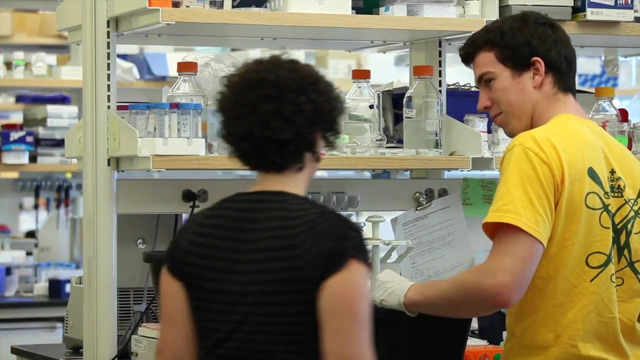 At some level. I think everybody is interested in finding a big discovery. The systems biologists are doing this in a way that relies very heavily on collaboration. Our lab would not be able to exist without collaboration. We collaborate with all these different investigators. 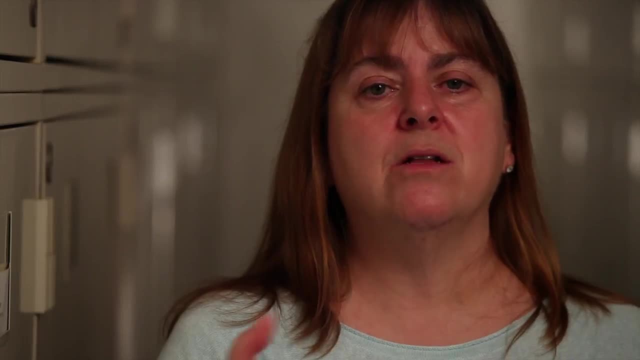 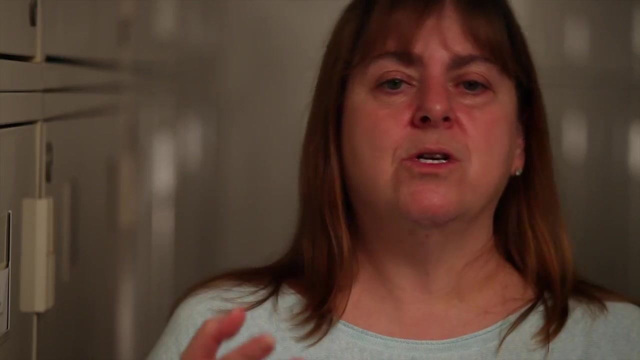 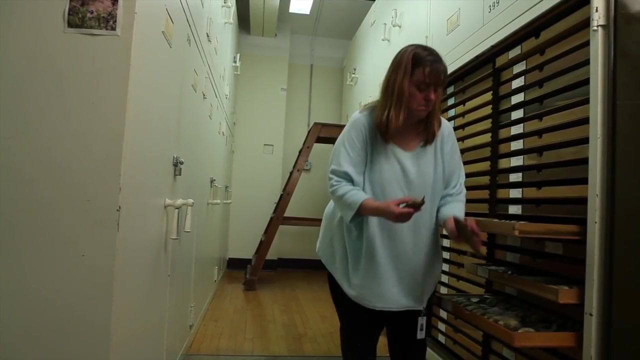 That's imperative for our work. I think that's the beauty of systems biology: is when you put people together who don't normally talk, all of a sudden, new possibilities arise from research and collaborations. In this century, systems biology is the way of thinking about the world. 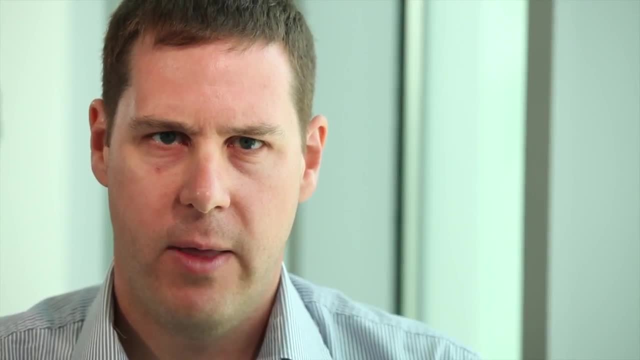 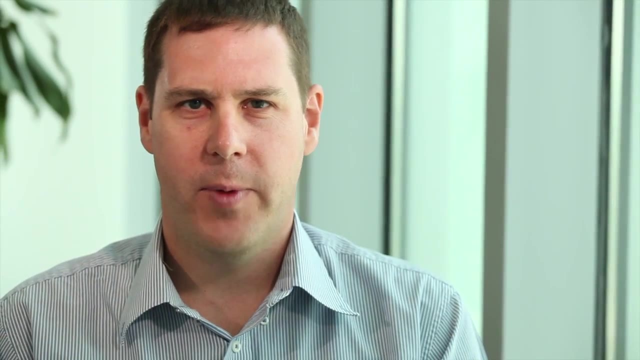 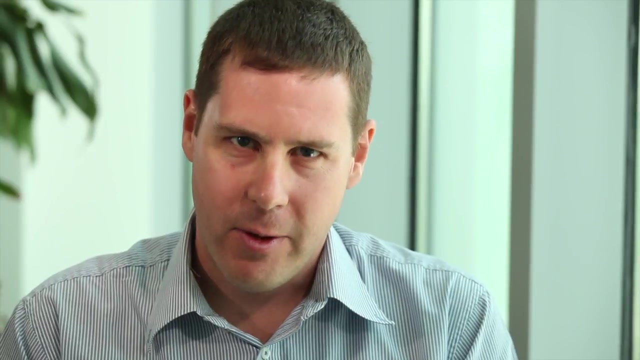 that's going to lead to those new discoveries and those new technologies. If you want to be a systems biologist, what you need to do is you need to learn math, You need to learn statistics, You need to learn a little bit about engineering. 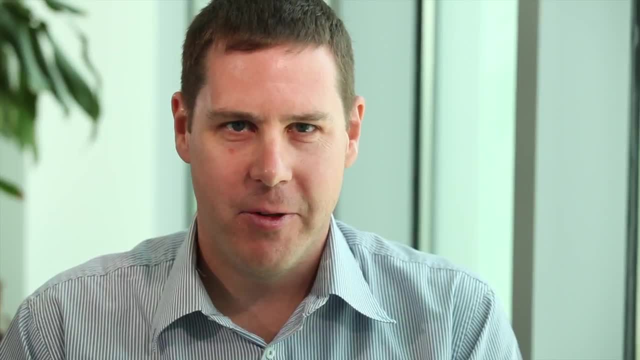 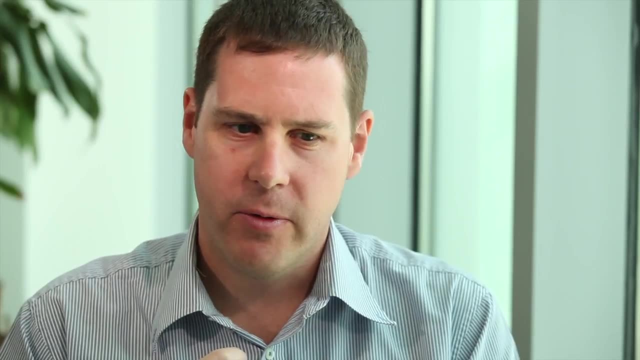 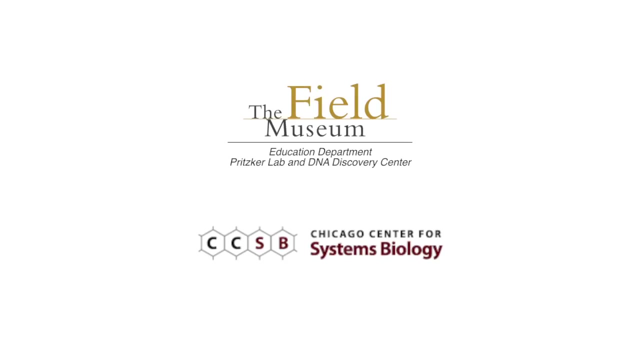 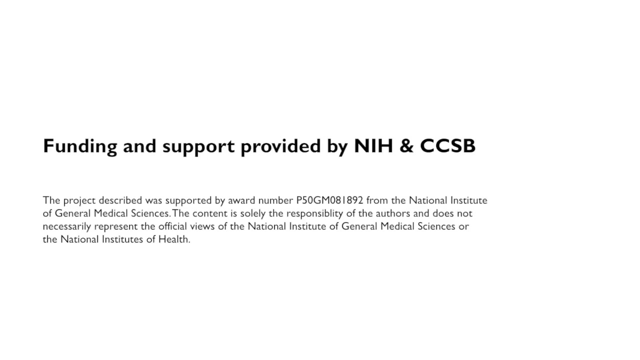 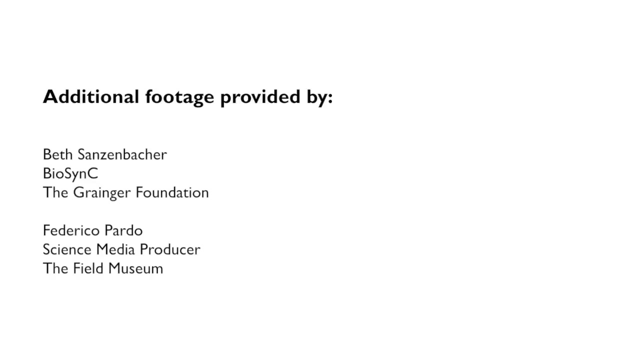 And you need to learn a little bit at least about biology. Once you have those tools, you can bring them together to attack problems in almost any area of biology that you find yourself interested in, And so I would bet that when you're in your 90s or 50s-